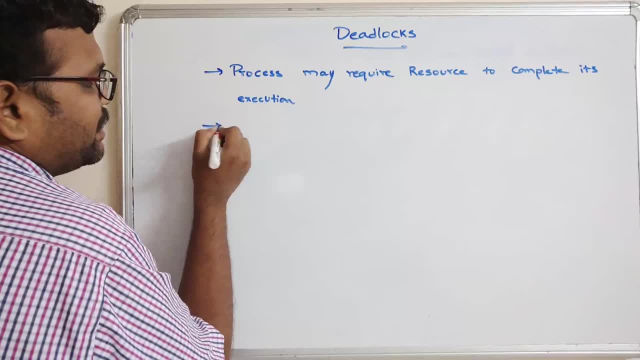 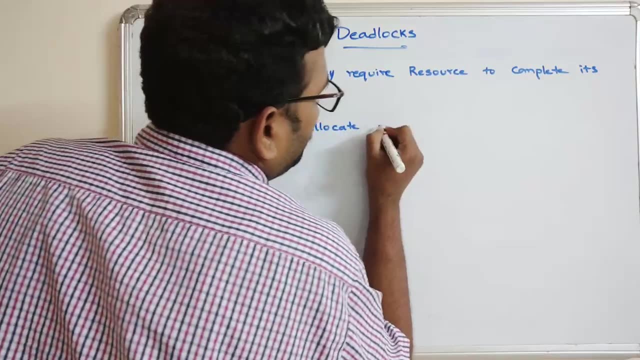 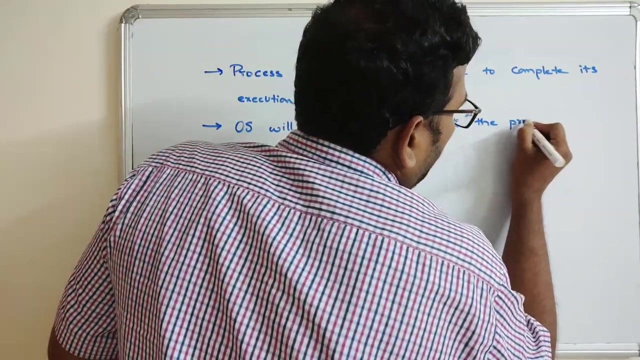 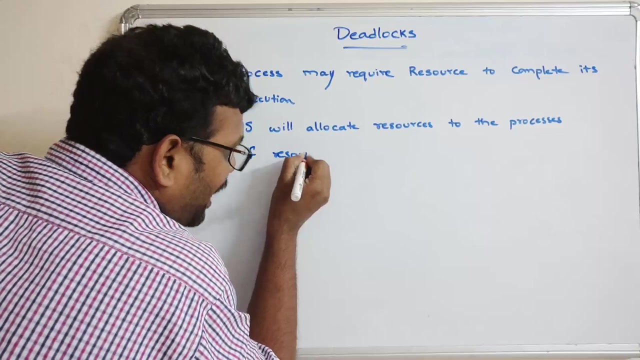 That's the first one. So once the work done by the process, automatically the resources will need to be got. So that is the first one Right. Next operating system will allocate resources to the processes. So the processes If resources are not available. 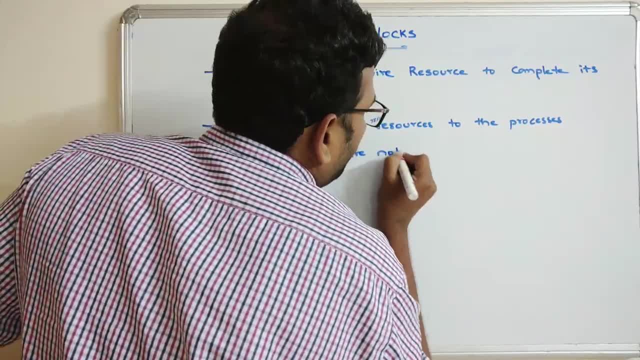 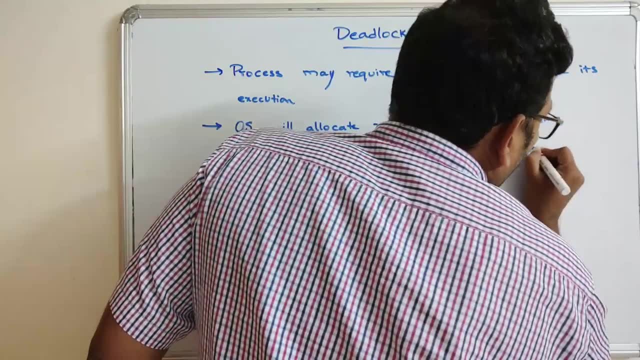 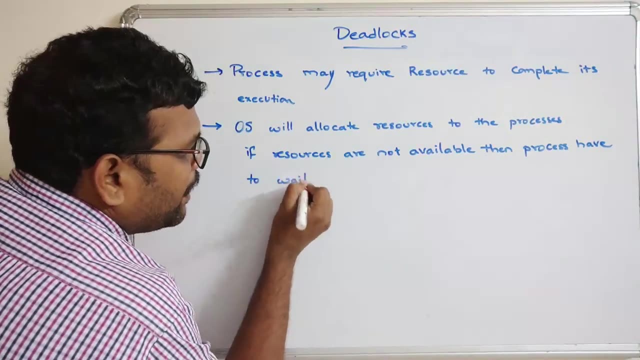 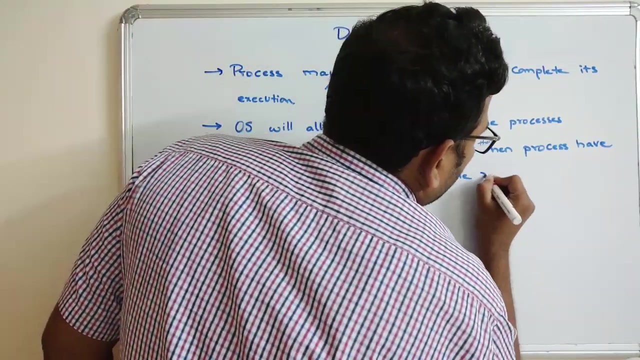 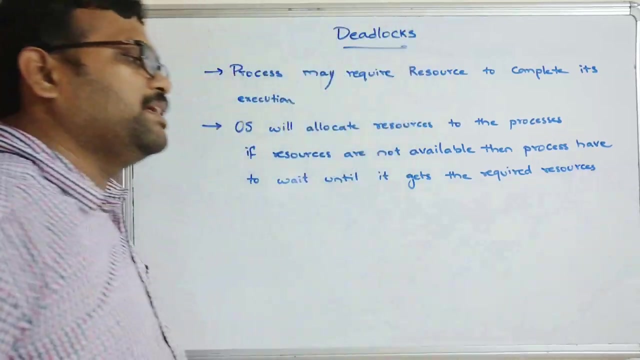 Resources are not available to the process, Such process may require resources. So if inf Breakdown the construction of a system- the instances represent the uses and works- then the process have to wait. the process have to wait until it gets the required resources. so required resources, so without the resources, the process will not be get executed if it requires. 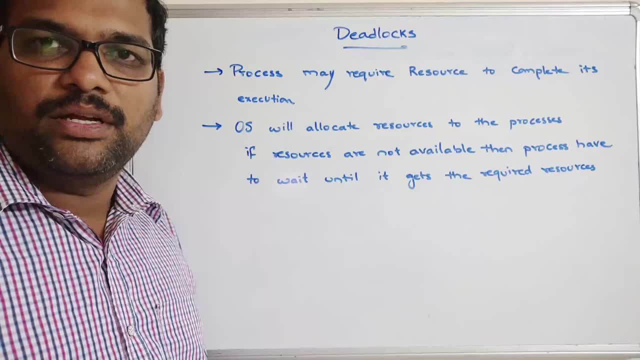 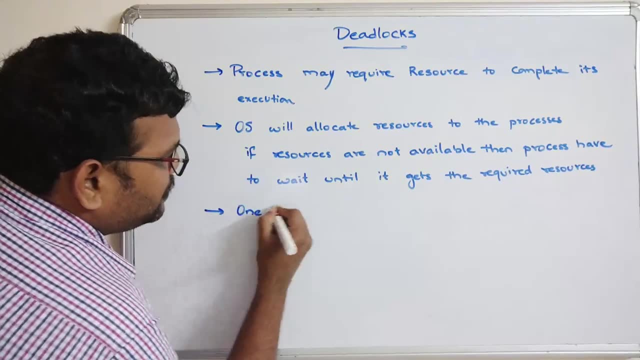 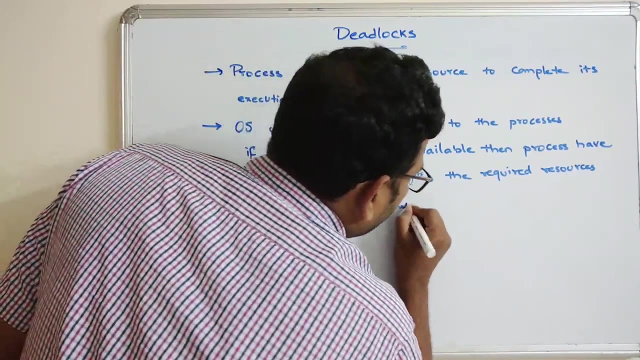 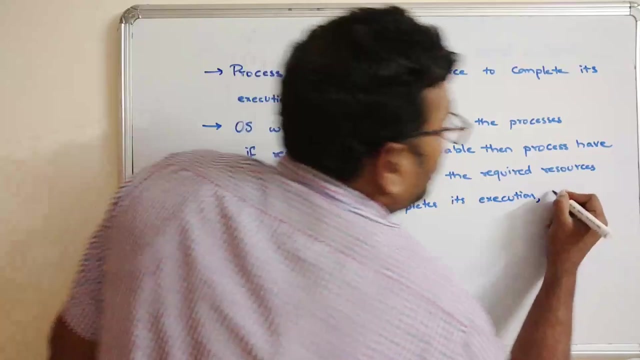 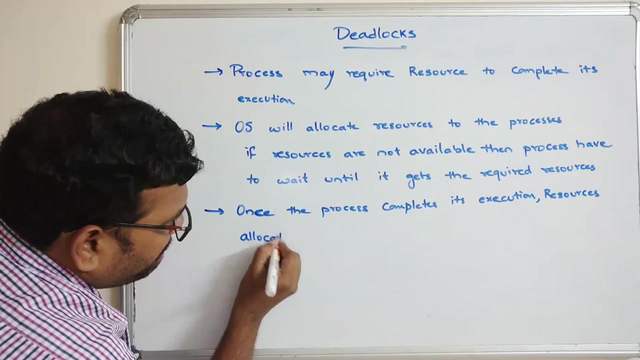 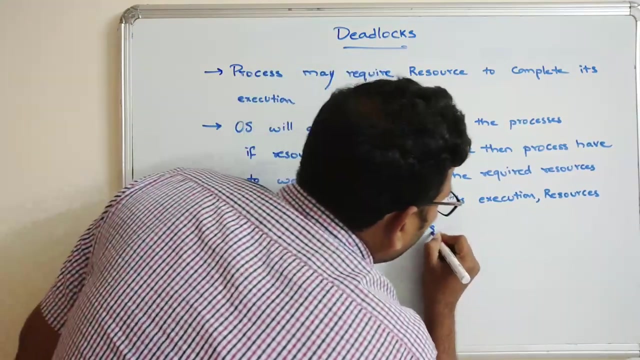 any resource, so it have to wait until it gets the resources. and all those resources will be allocated by the operating system itself and the next one once the process, once the process completes its execution, completes its execution, resources, resources allocated to that process, should be released. should be released, that means whatever the 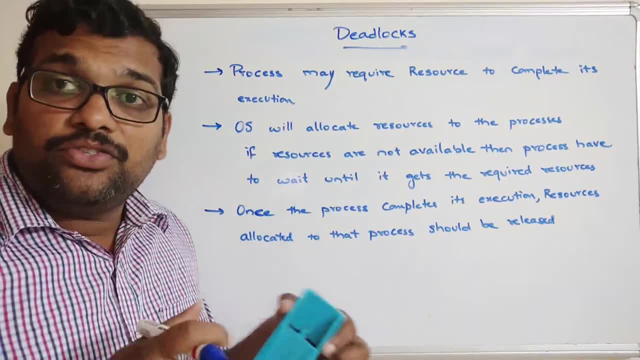 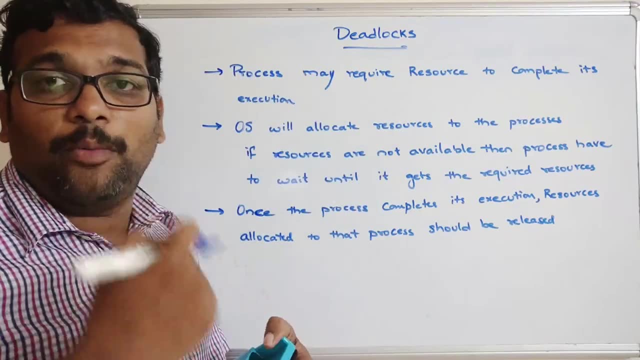 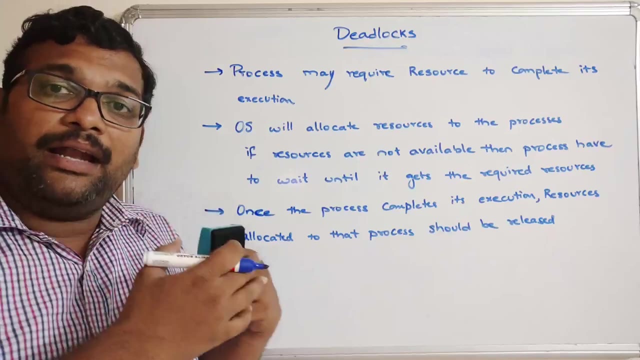 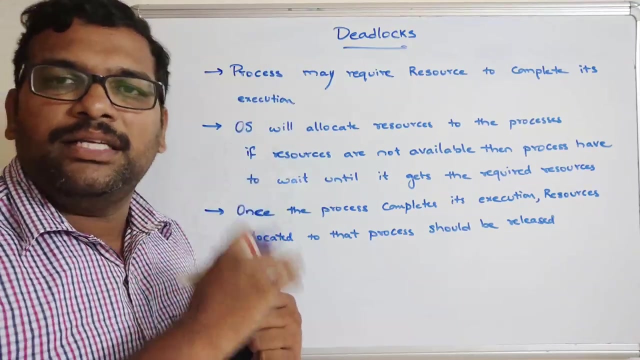 resources which are allocated for that particular process should be released, the deallocated, so that those resources may be used by another process. so the operating system, immediately the operating system will find out the resources which are available and the operating system will allocate those resources to the corresponding process which are requiring these resources, right? so 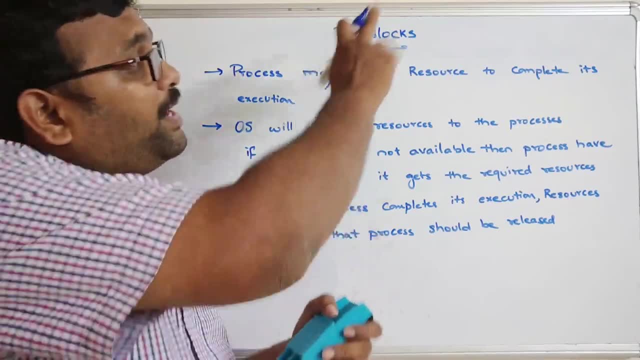 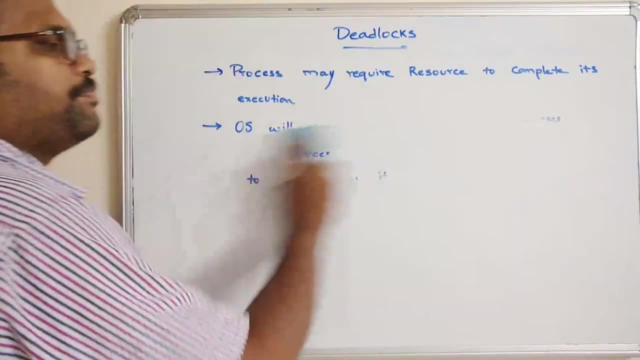 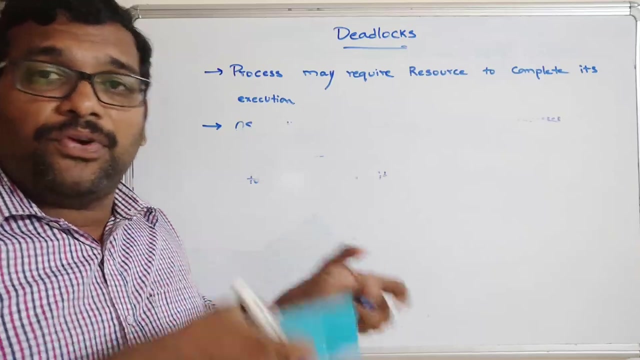 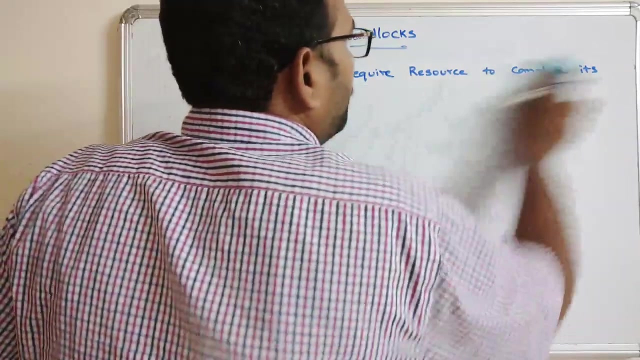 this is the steps going on right now. what is a deadlock? what is a deadlock? so? a deadlock is a situation. so it is a situation where one or more processes are being executed and waiting for the resources which are being allocated for another process. right see, I will explain so this. 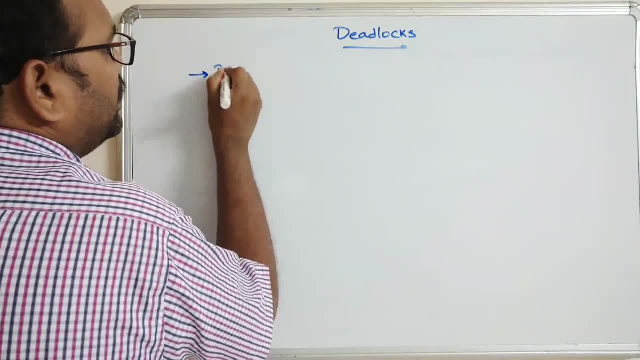 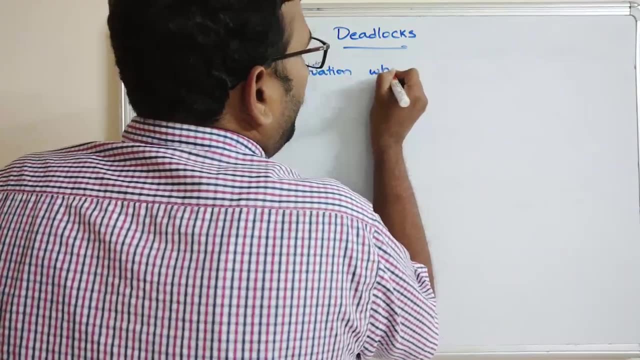 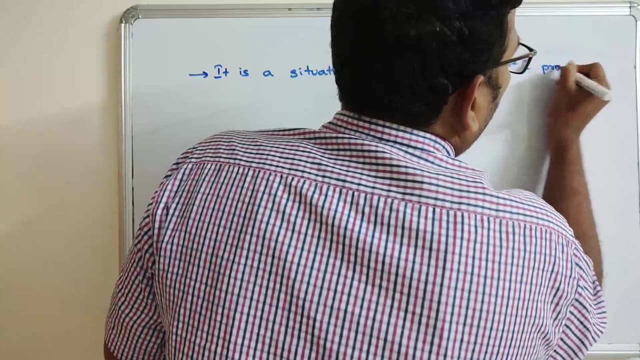 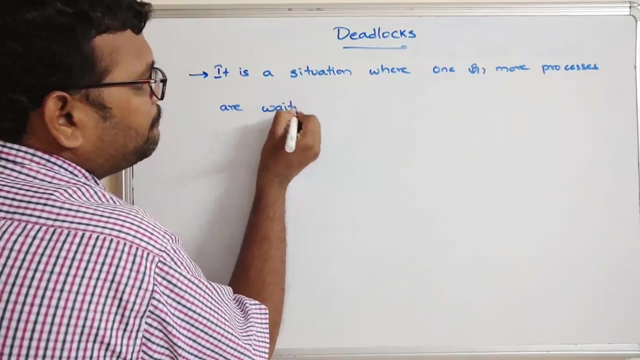 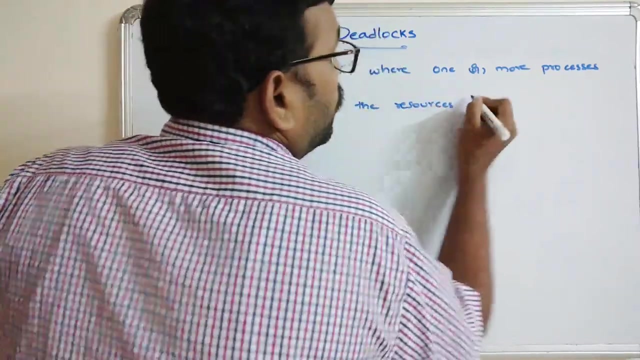 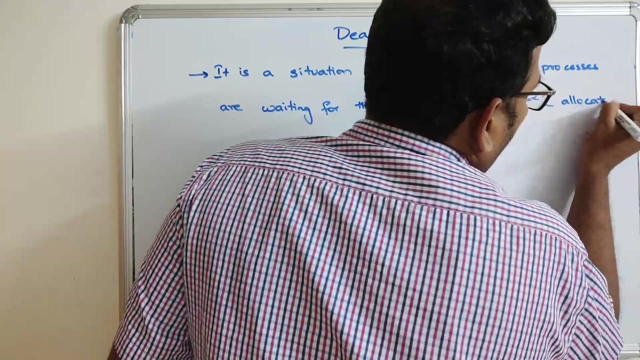 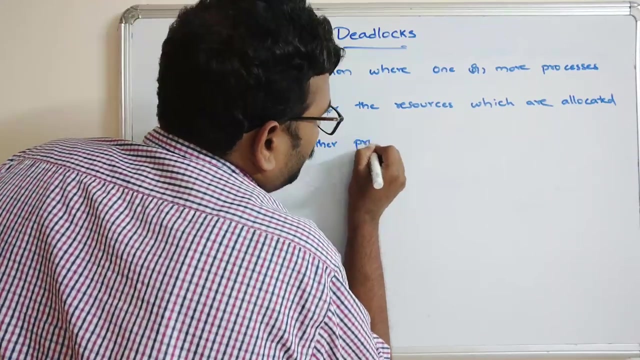 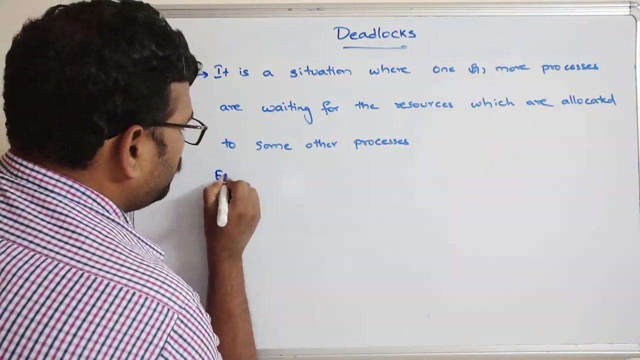 is a situation, a deadlock. it is a situation where one or more processes, one or more processes are waiting for the resources which are allocated to some other process, some other process. right, so example Let us take. so let us explain you with an example, so that you can understand what exactly the deadlock. 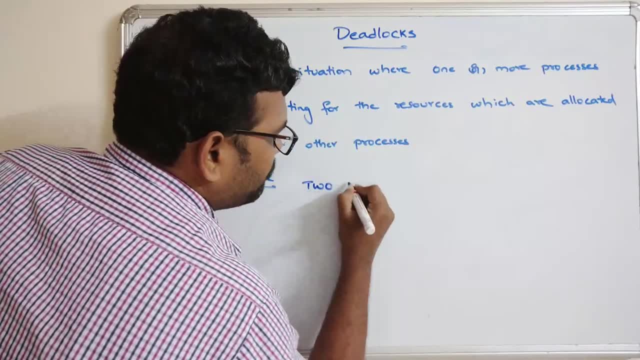 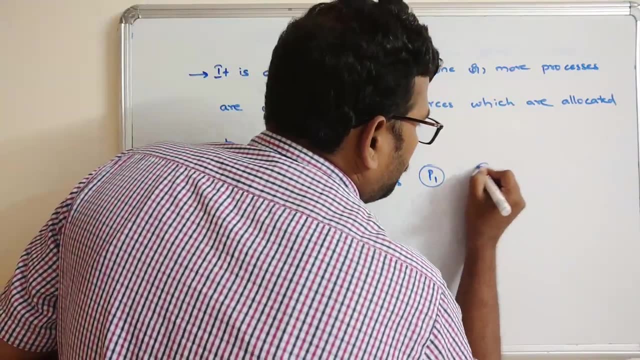 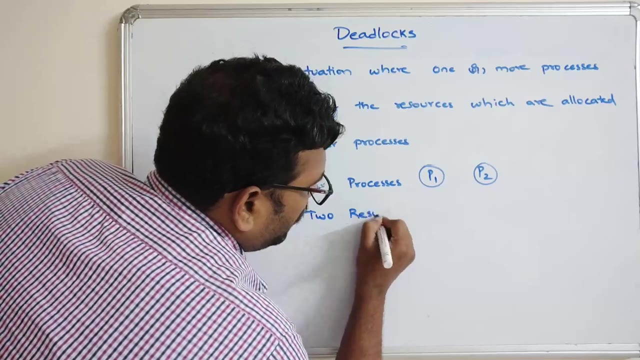 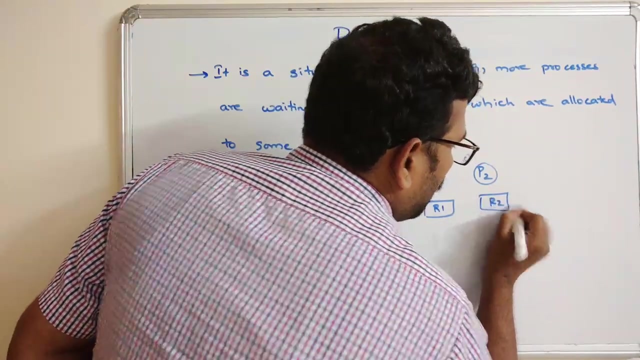 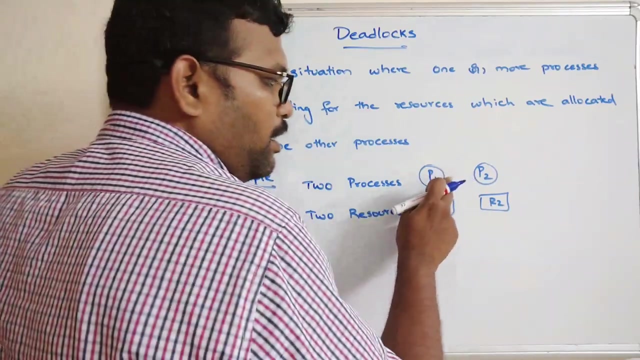 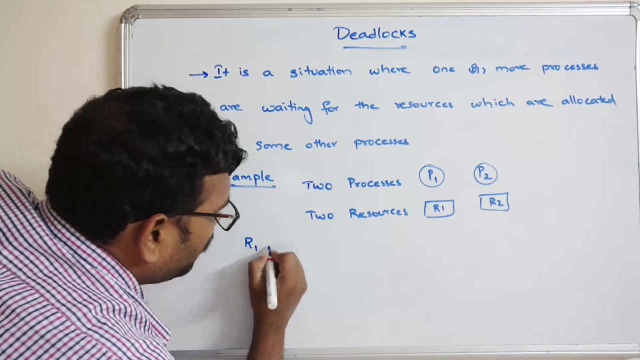 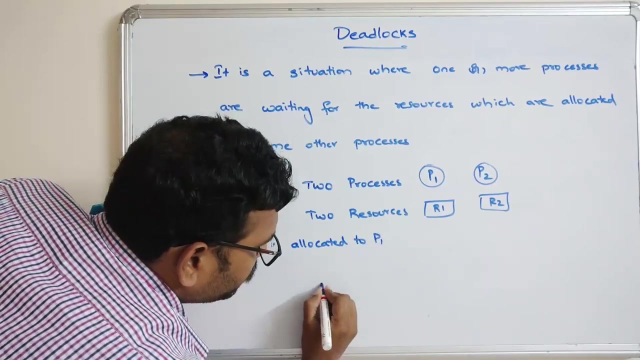 So let us consider two processes, two processes: P1, P2.. There are two processes and there are two resources. There are two resources. we call it as R1, R2.. Okay, two processes and two resources. So if P1 requires, I mean R1 is allocated to P1.. So I will write here: R1 is allocated to P1, right? So R1, which is being allocated to P1. 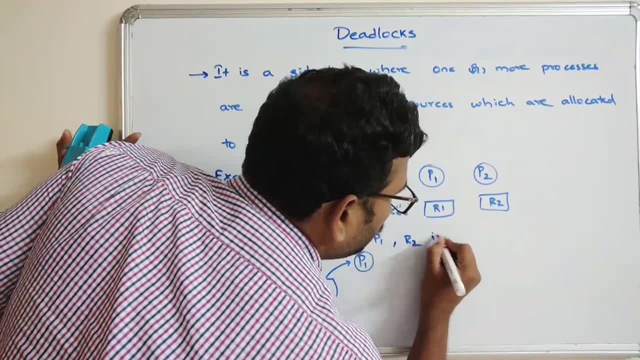 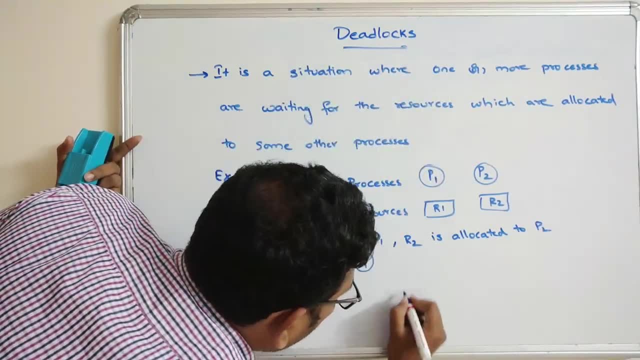 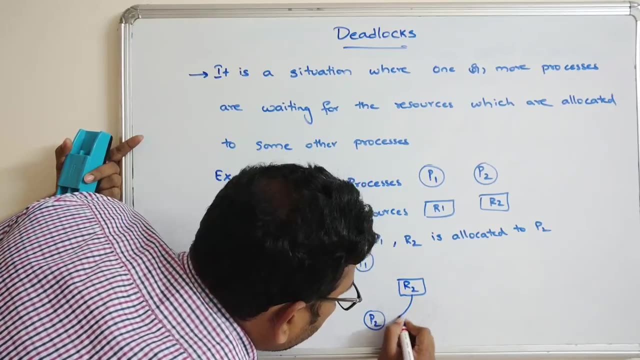 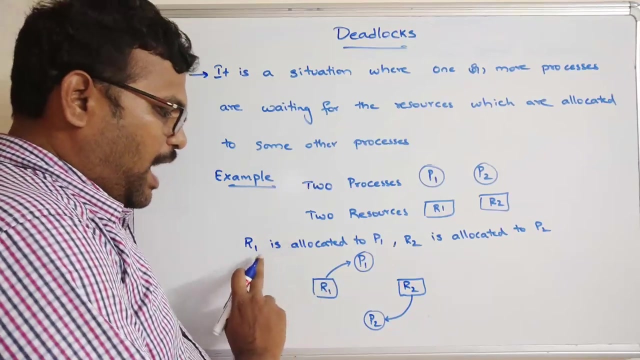 Similarly, R2 is allocated to P2.. So let us take here R2, which is being allocated to P2, right, So two processes and two resources. So if R1 is allocated to P1, that means a resource 1 is allocated to process 1 to complete its execution. 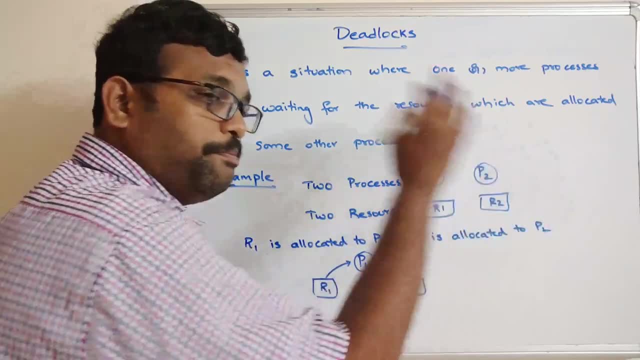 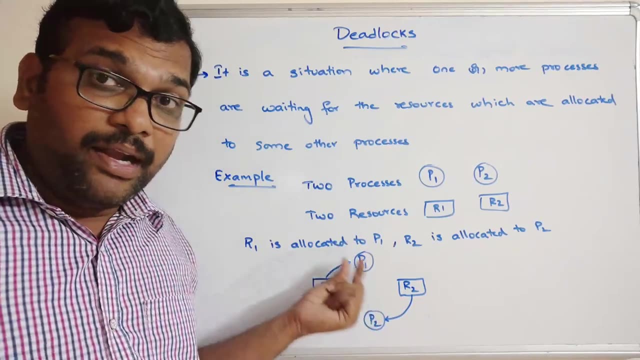 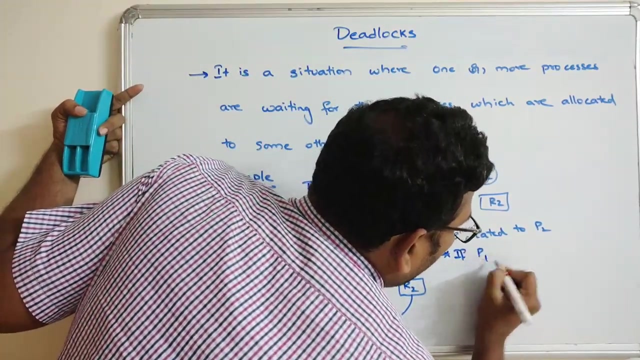 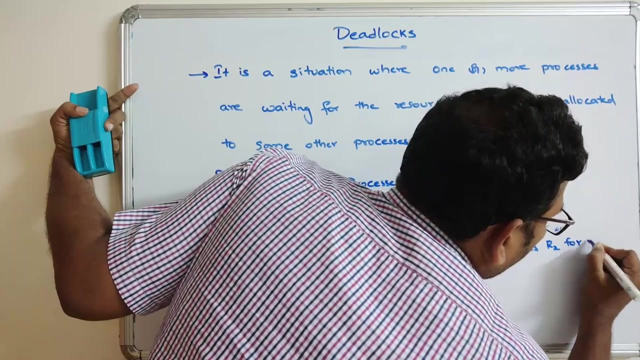 Similarly, R2, resource 2 is allocated to process 2 to complete its execution. So, in order to complete the execution of P1, if it requires R2, right See- I will write here If P1 requires R2 for its completion. 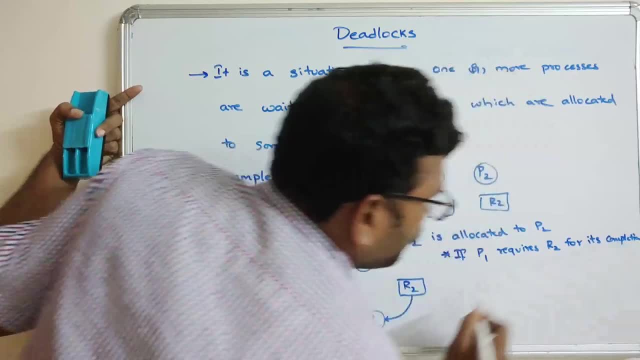 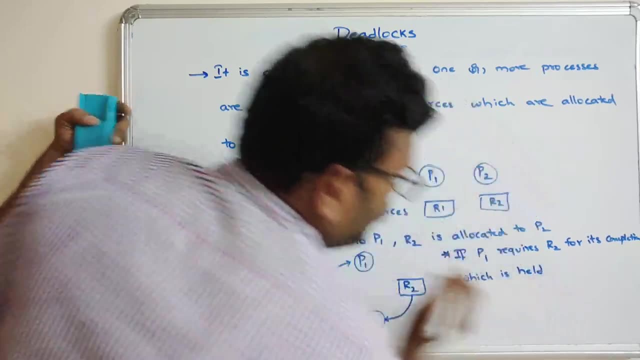 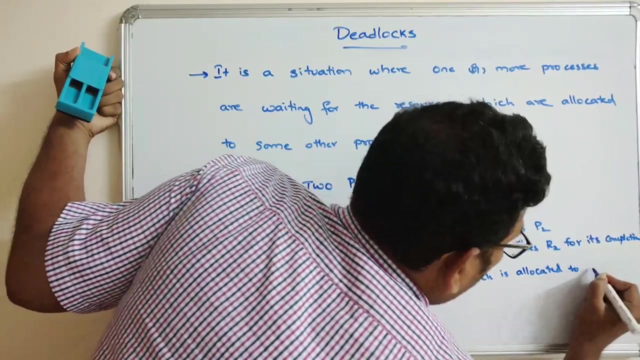 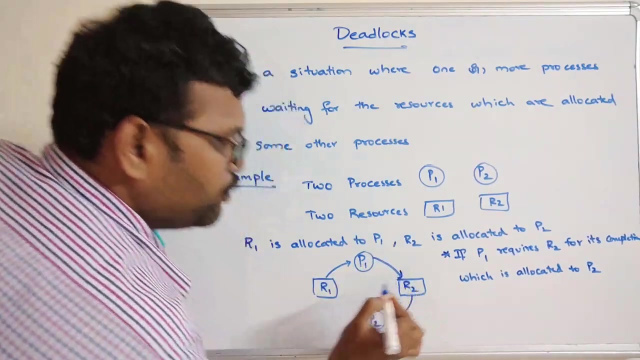 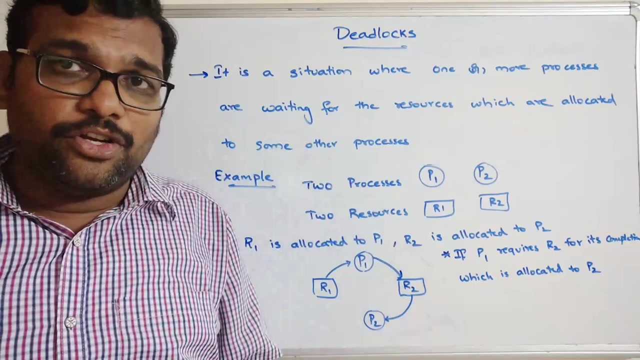 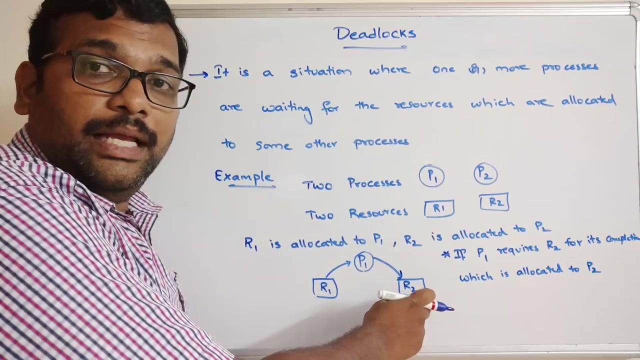 which is which is allocated to P2.. That means P1 is requesting for R2 to complete its execution. That means P1 requires already R1 is allocated to P1. But in order to complete its execution, P1 requesting the resource R2.. But here what happens? R2 is allocated to P2.. 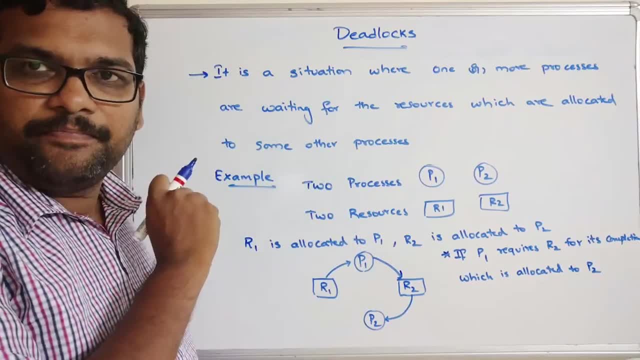 So, SO, P1 will be in a waiting state, But in order to complete its execution, P1 is allocated to P2.. OK, so, which is allocated to P2.. Okay, so, which is allocated to P2, If similarly, the second point. 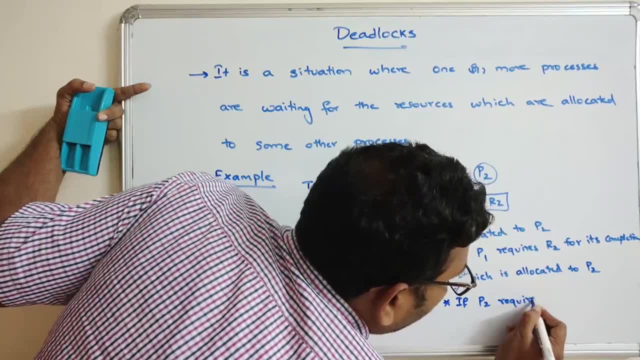 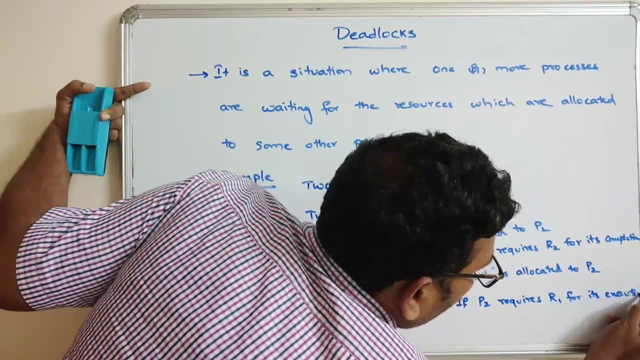 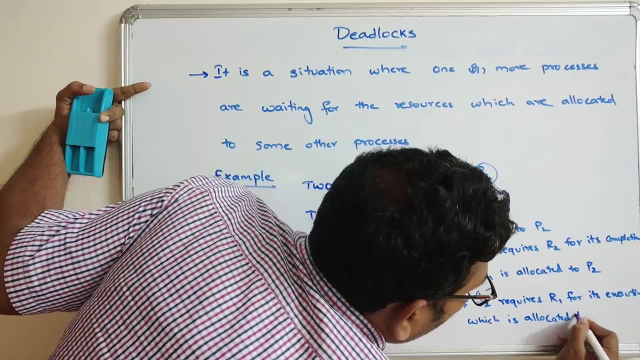 if P2 requires R1 for its execution, for its execution, which is allocated to P1.. which is allocated to P1.. So P1 requires too R1.. So P1 requires too R1 for its execution. so which one requires for their execution. So R2, the first thing that we have to know is that For all other processes of execution, is there annung to R2 as well as 32 to R1 is allocated 2, all 3 processes to component, then there is no limitation, which is allocated to P1 and which measure R1 and RN is allocated to P2.. P2 requires R1 in order to complete its execution. P2 requires R1 to complete its execution, which is allocated to P1. So P2 will be also in the waiting state. So because in order to complete the execution of P1, it requires R2.. R2 is already allocated for P2.. So P1 has to wait. 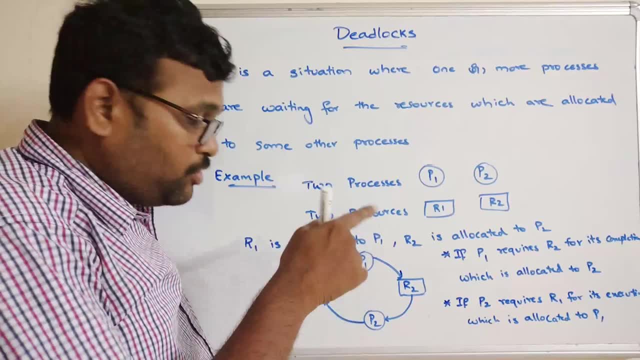 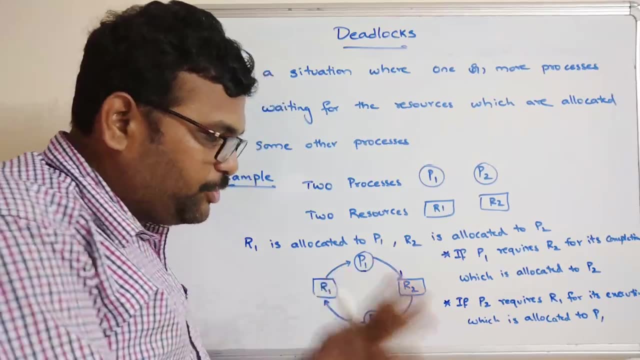 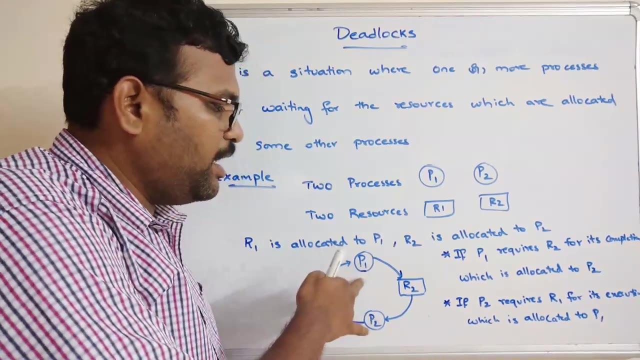 until P2 releases the R2.. So P2 will release the resource 2 whenever it completes its execution. But here, if the situation is like this, that means if P2 requires R1 to complete its execution, which is allocated to P1. So P2 will be in the waiting state until it receives the R1. 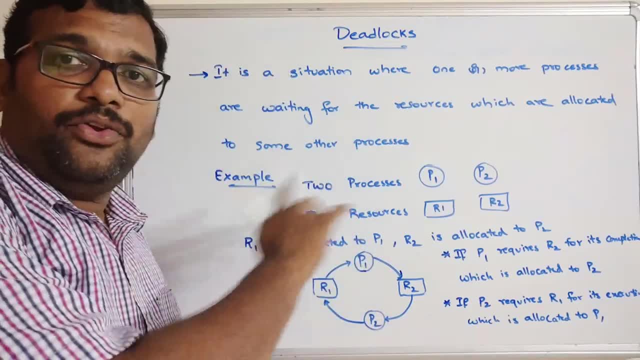 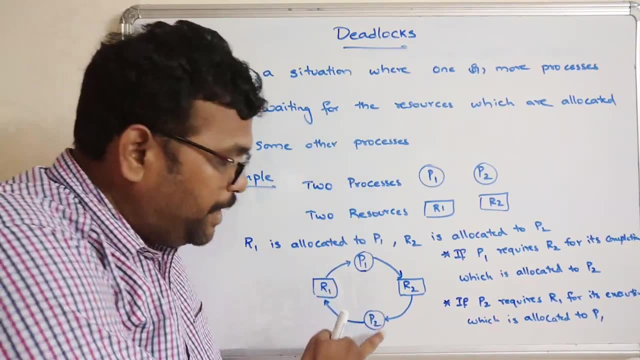 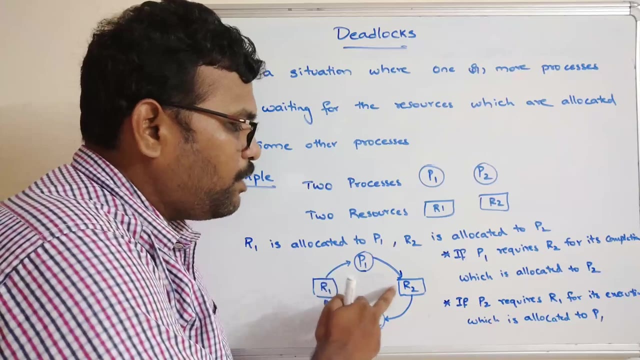 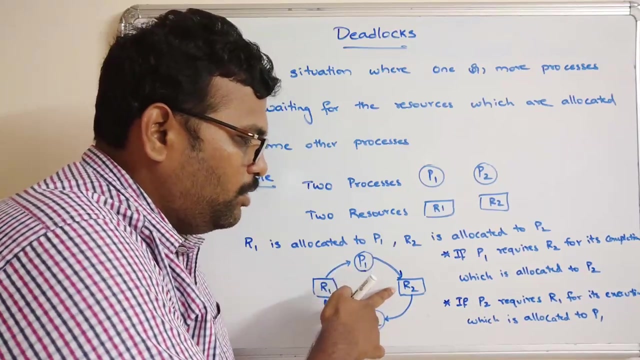 which has to be released by P1. So here you can observe the situation: P1 will release R1 only after its execution, P2 will release R2 only after its completion of execution. But P2 requires R1, P1 requires R2.. So unless the P1 gets the R2, P1 will not complete its. 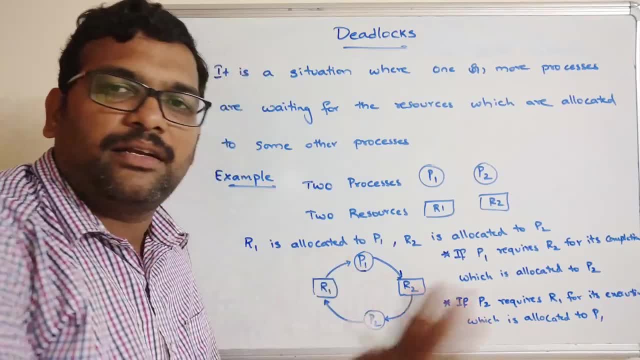 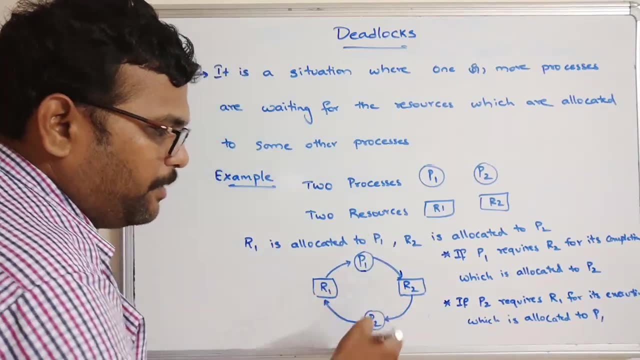 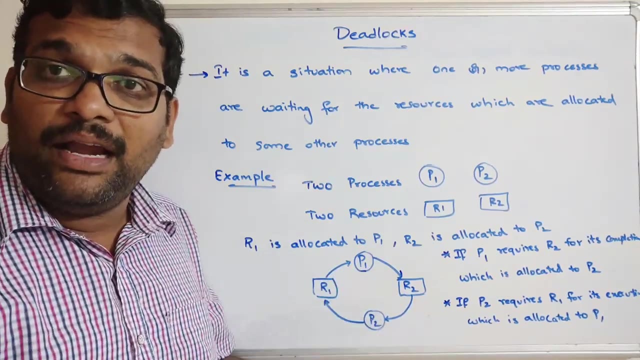 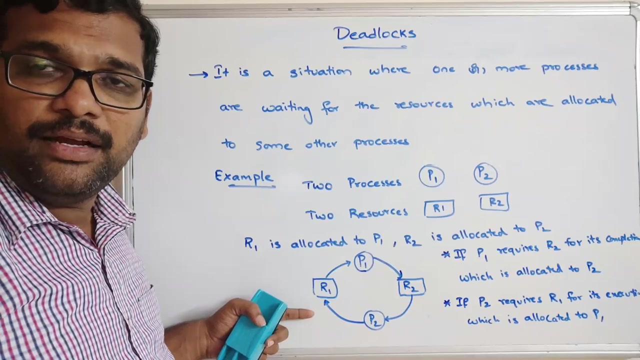 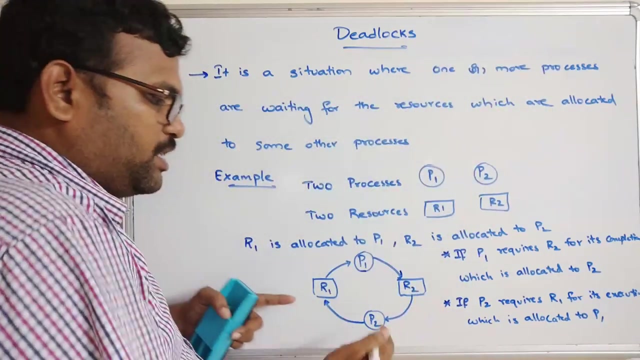 execution Until P2 gets R1, P2 does not complete its execution. So this chain process. so here, in this situation, P2 will release R1 only after its completion of execution. So unless P1 and P2 will be in the blocked state, so both will be in the waiting state. so this is a never ending process. so such a situation we call it as a deadlock. such a situation we call it as a deadlock situation, right? so it's a situation where one or more processor waiting for the resources. so here P2 is waiting for R1, P1 is waiting for R2, which are allocated to some other process. 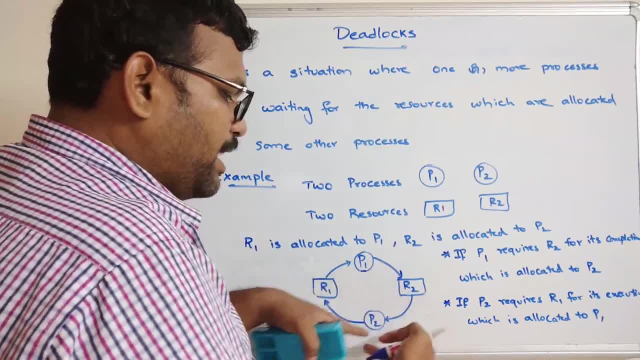 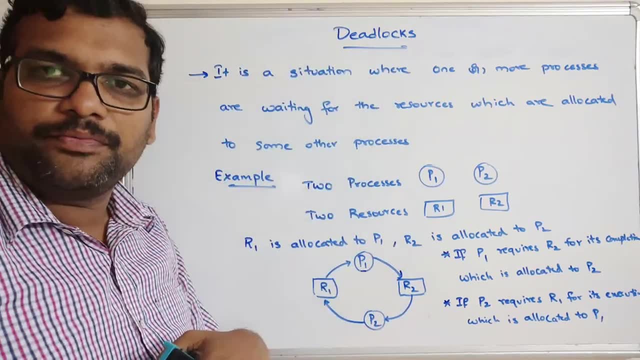 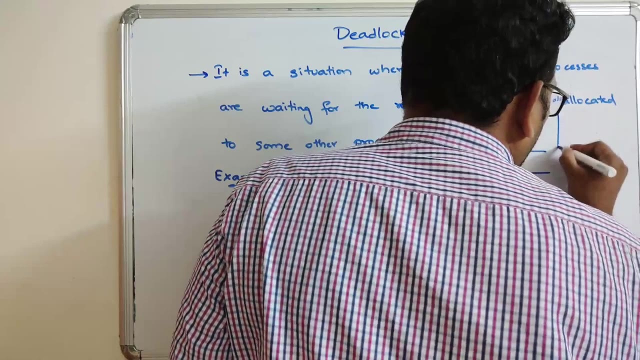 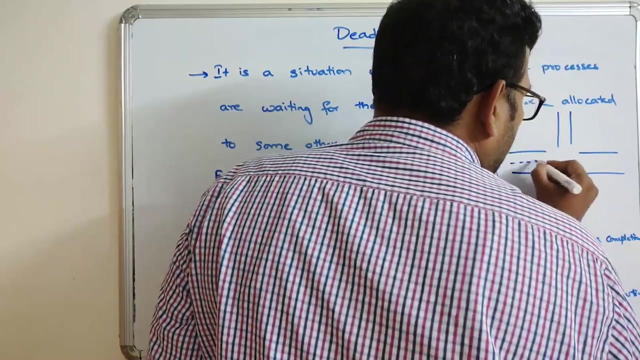 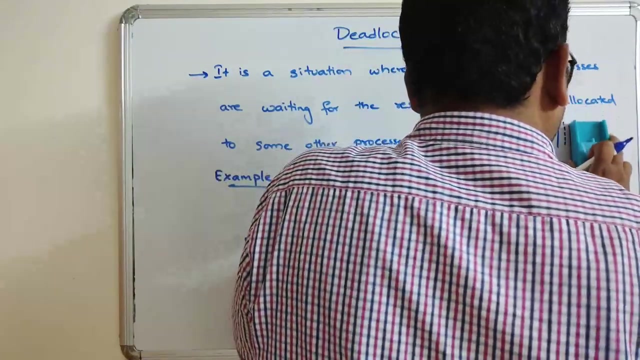 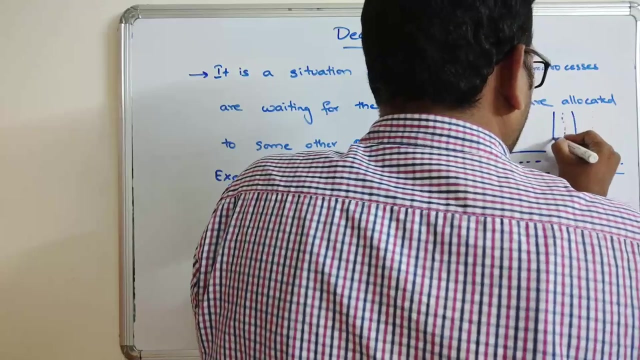 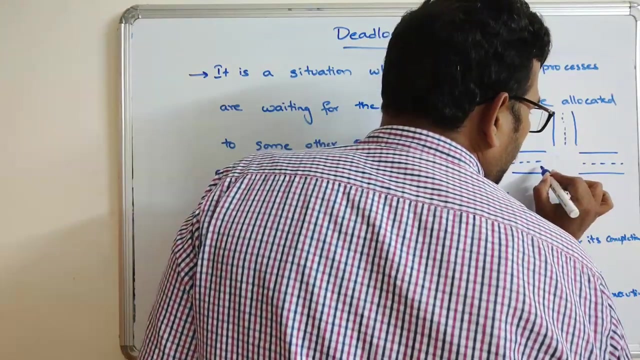 so R1 is allocated to P1, R2 is allocated to P2. so this type of situation we call it as a deadlock situation. deadlock situation. so just for understanding, I will give you an example. so traffic, traffic, right, see, let us take this is a oh so. so there is a center, okay, where this is a center, right. so if car from this side wants to move here, ok, and car move here, and car gets here, and car gets here. 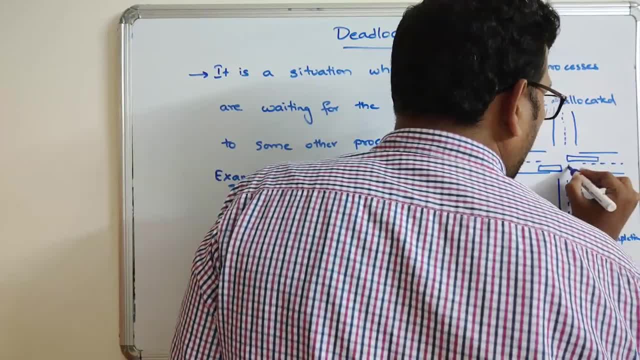 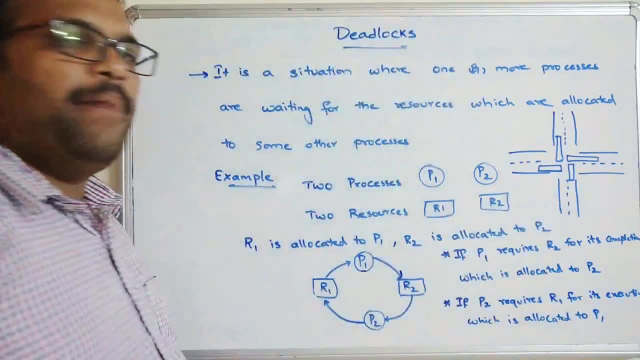 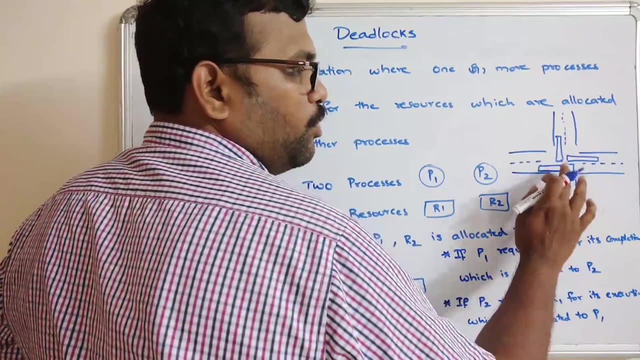 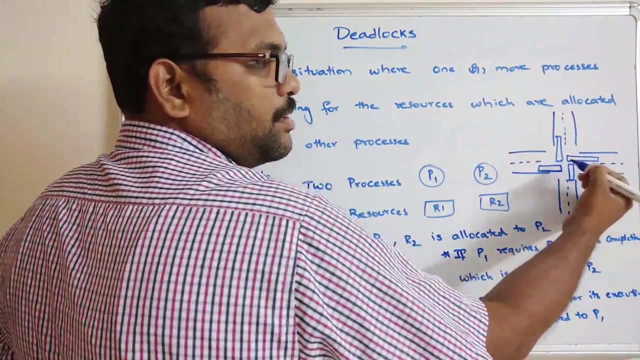 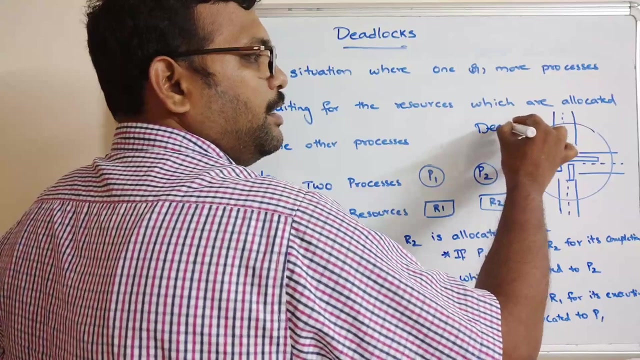 here, ok, and carbose here, and other students here, and targets here. you can see, Imagine this situation. So this car, this car wants to move this side. So when it will move, Whenever this car moves towards a friend, it will move. So this is struck, This car is struck, This car is struck. So such a type of situation is called as a deadlock situation. 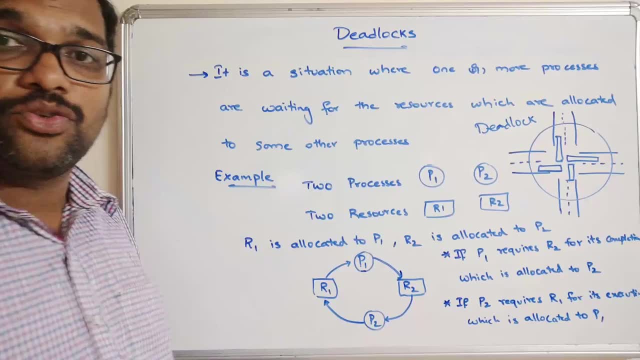 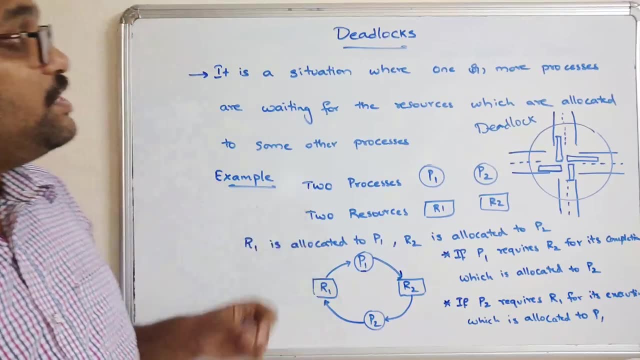 Such type of situation we call it as a deadlock situation. So here what happens? All the cars will be in the waiting state. This is a never ending process. Okay, So such a situation we call it as a deadlocks. Such situation, we call it as a deadlocks. 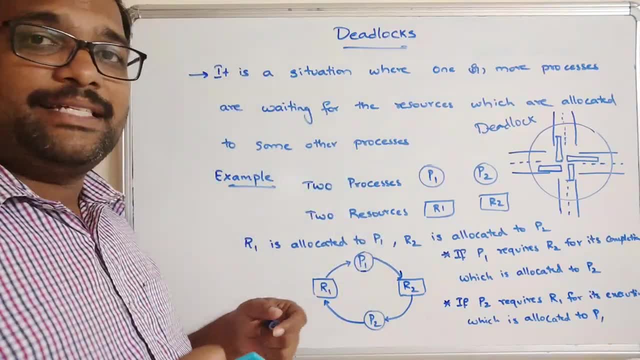 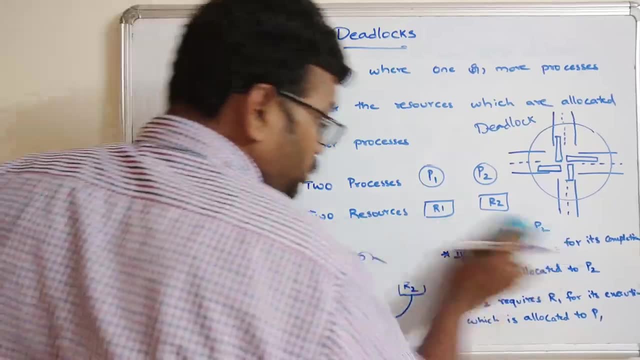 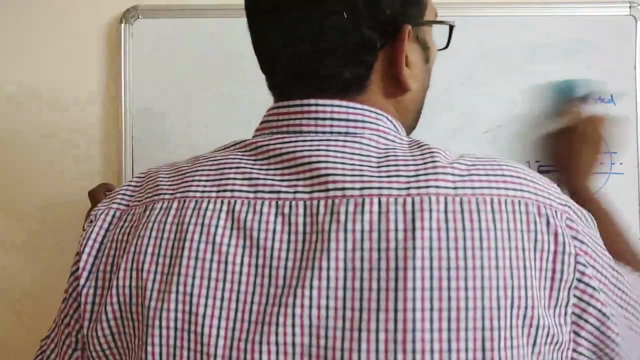 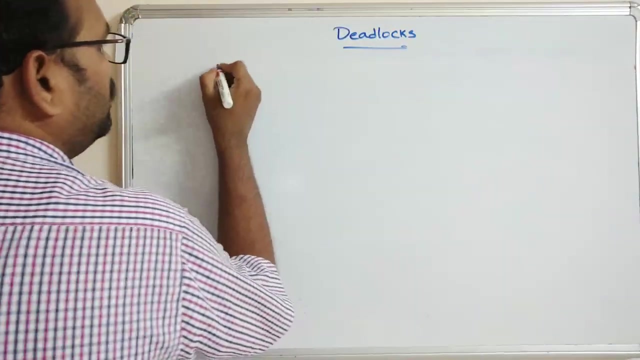 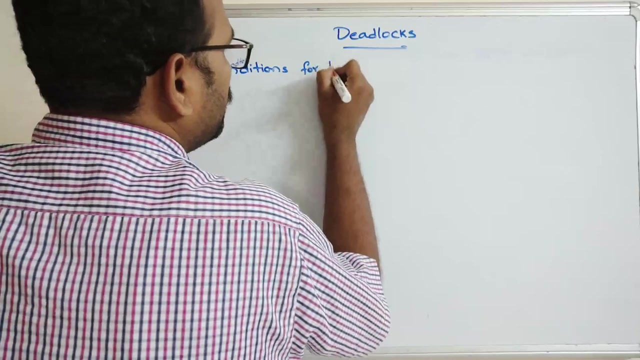 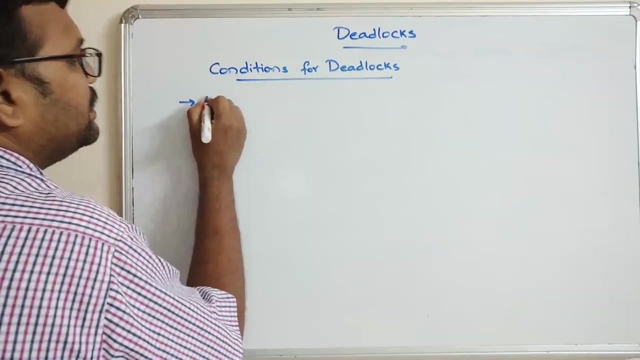 And now we will see what are the necessary conditions that to be satisfied, if the situation is a deadlock, That gives a deadlock situation, That makes a deadlock situation Right. So conditions For a deadlock, What are the conditions for deadlock? So there are mainly four conditions for a deadlock situation. So conditions for deadlocks. So first one is a mutual exclusion: exclusion, Mutual exclusion. 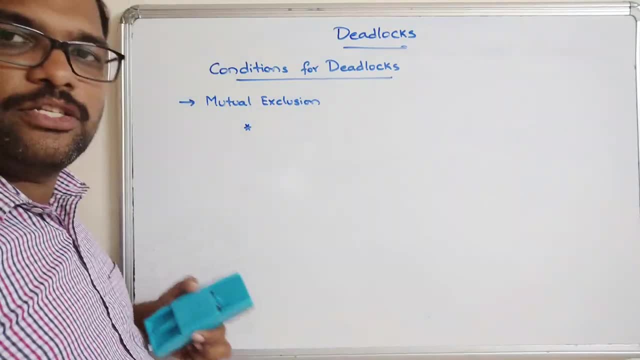 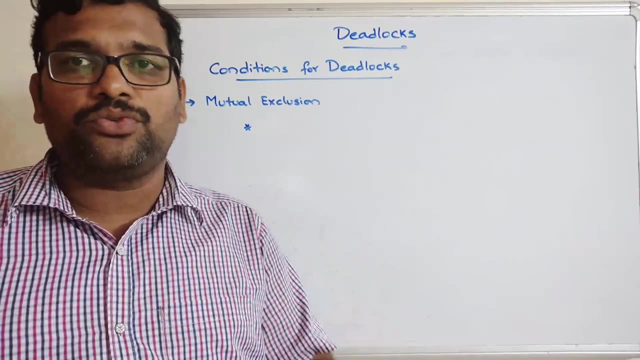 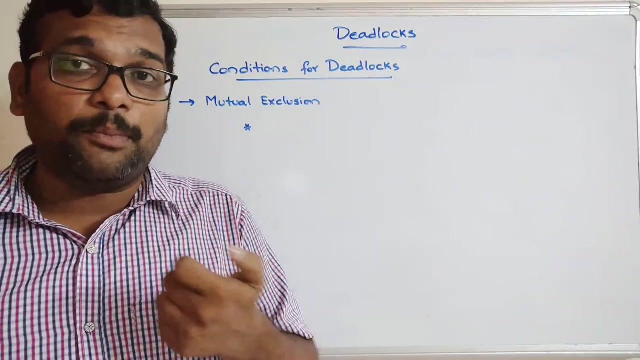 So this already we have discussed in our previous sessions. Mutual exclusion means so if one or more process wants to share the resources at a time, only one process should share it, Right? So if one process is allocated- I mean one resource is allocated to one process, So other process have to wait until completes its execution- That we call it as a mutual exclusion. 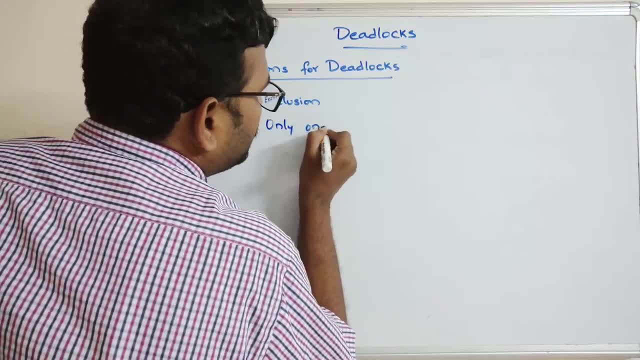 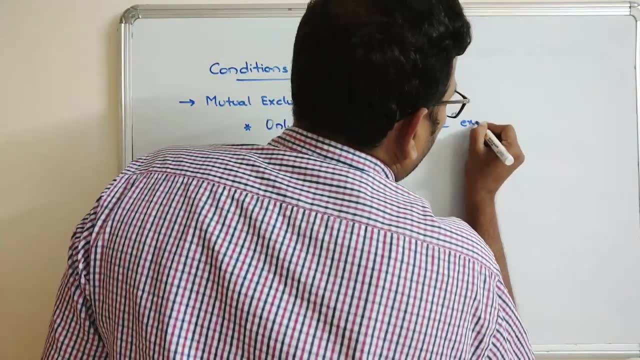 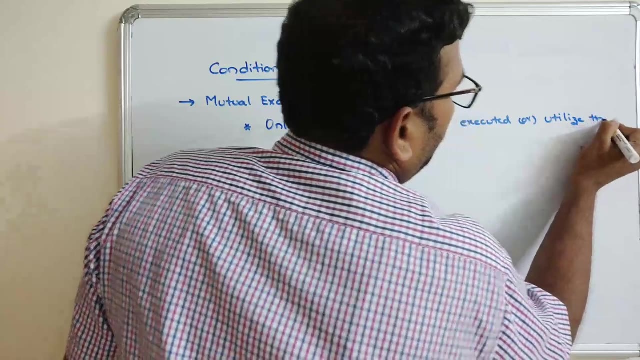 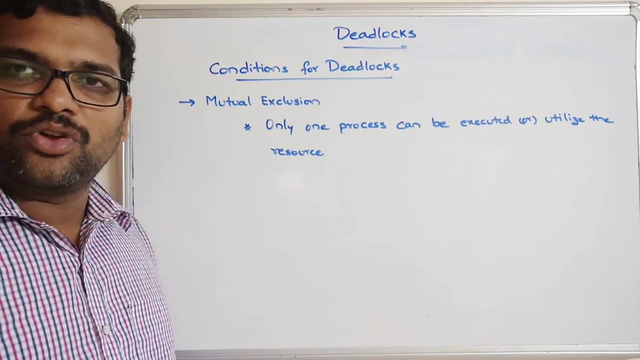 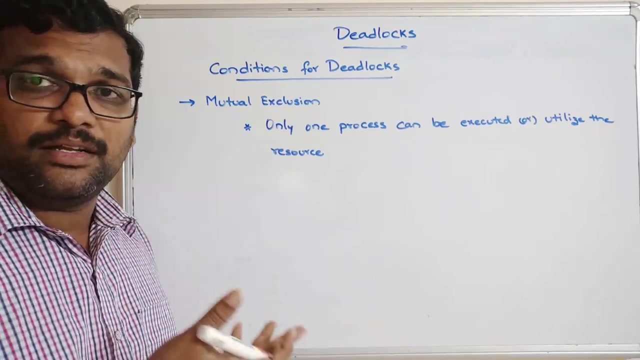 So only one process And be executed or utilize the resources. So only one. one process should recTrax resources, So other process have to wait, Right. So this is one reason why we are getting the deadlock, because if one process, like, for example, or one, is allocated through P, one example are one is allocated to open worked and 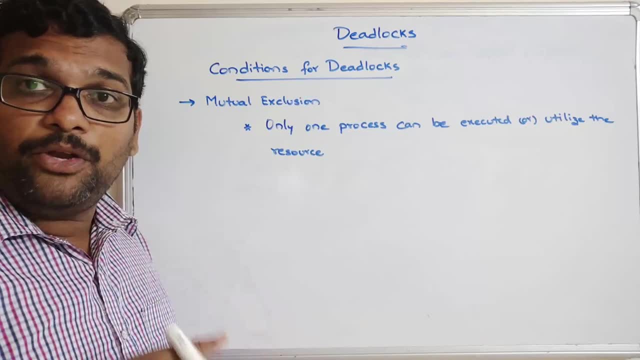 In our previous example, Or one is allocated to right, Like in case of a 1, x, S, 1. Of purpose to P1 and P2, have to wait until the P1 releases the R1 so that we call it as a. 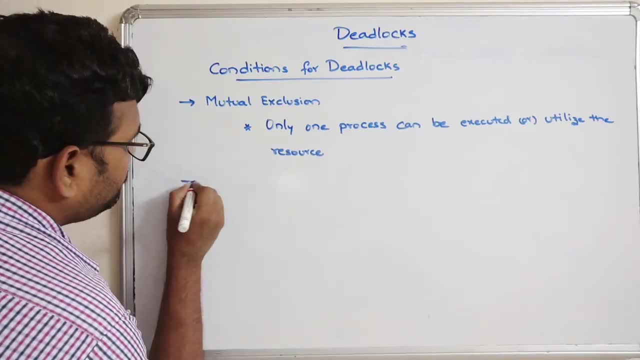 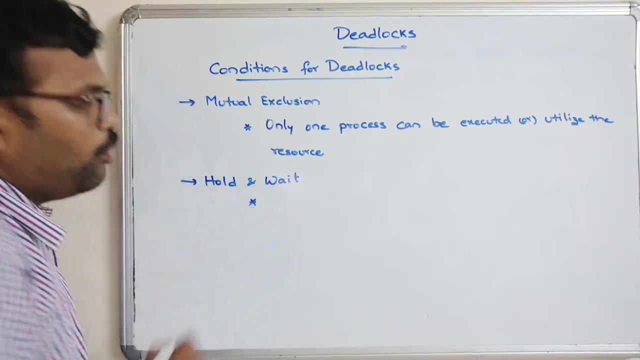 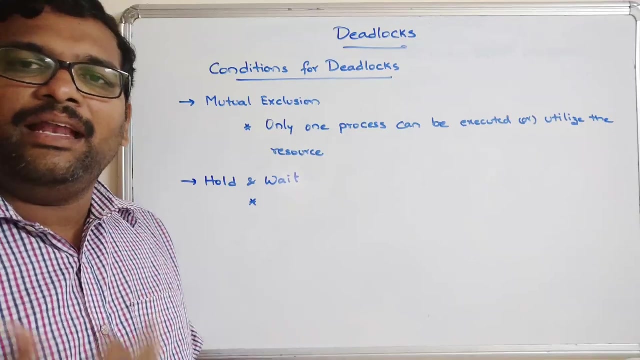 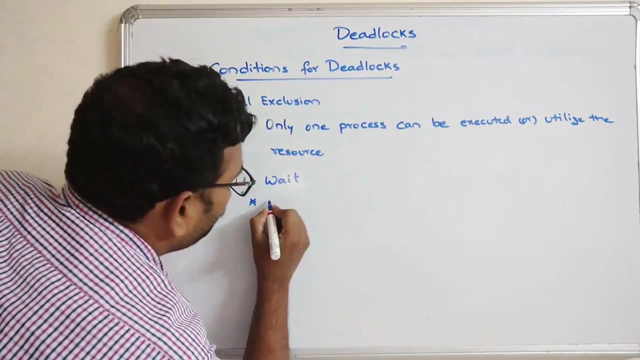 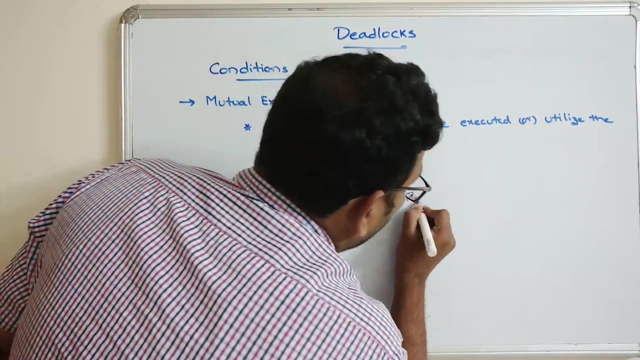 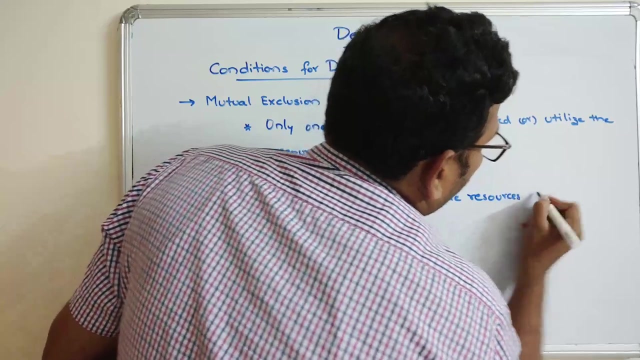 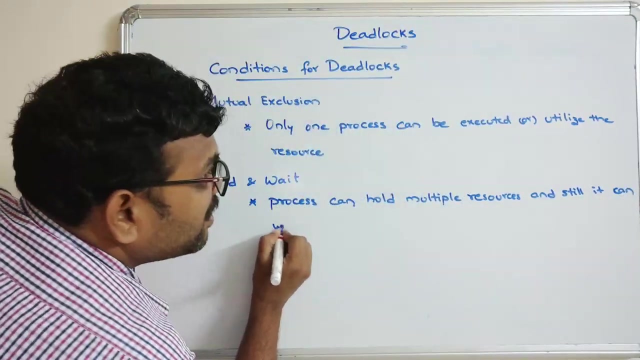 mutual exclusion. the next one: hold and wait. this hold and wait means one process can hold multiple resources and again it can wait for any other resources. right, so one process can be availing multiple resources. so a process can hold multiple resources, multiple resources, and still it can wait for. 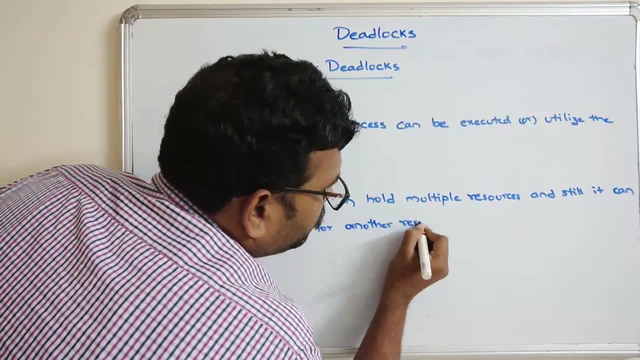 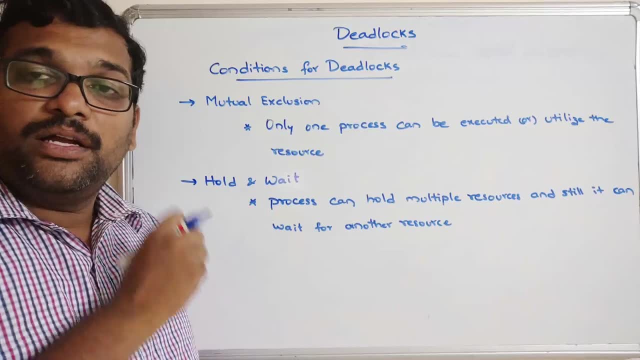 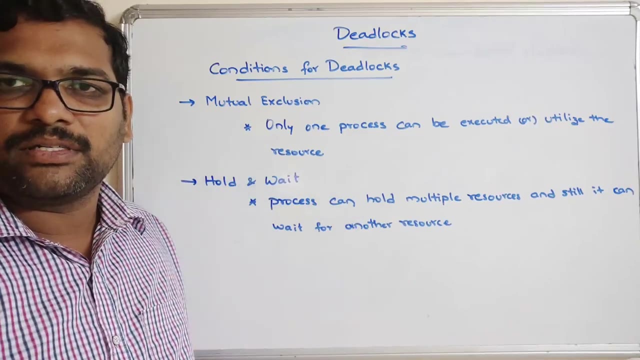 I: Another resource, Another resource. So if the process want to release the resource, it should get another resource and then only it can complete the process and it can release the resources. So this is the second condition why we are getting this deadlock situations. 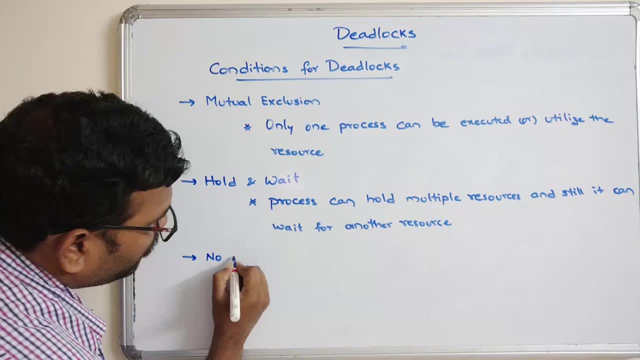 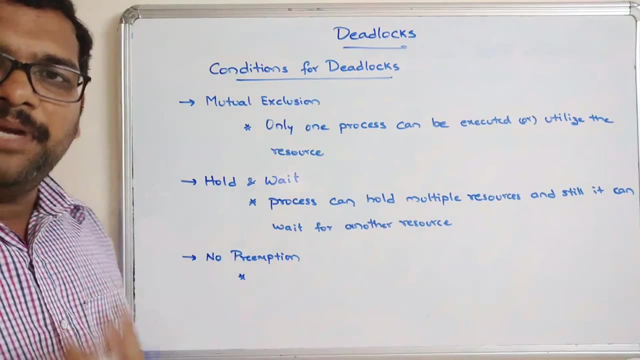 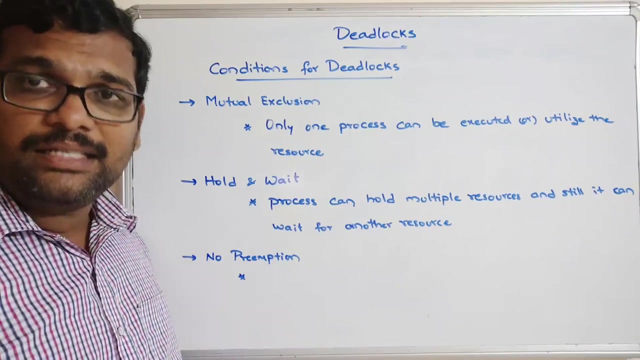 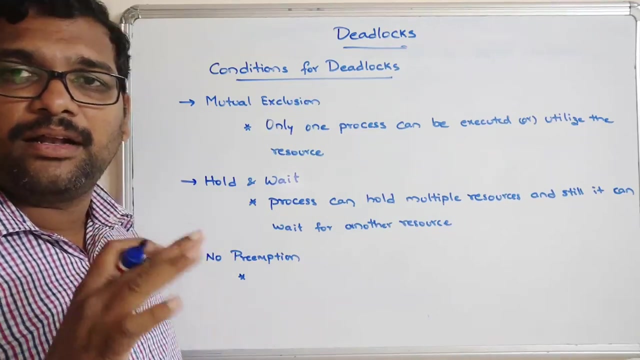 And the third one: no preemption, No preemption. So here, no preemption means so no interruption. So the process have to release the resources only after the completion. So the user of the operating system can't release the process by force, I mean can't release the resources from the process. 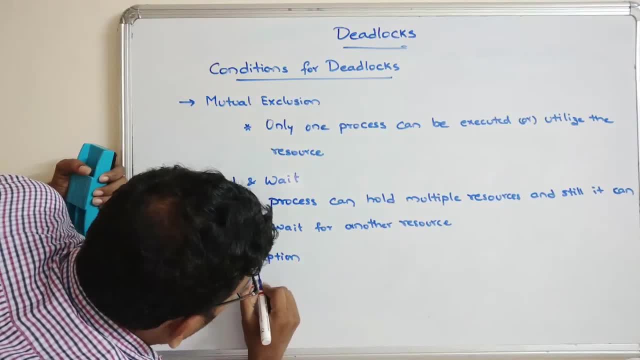 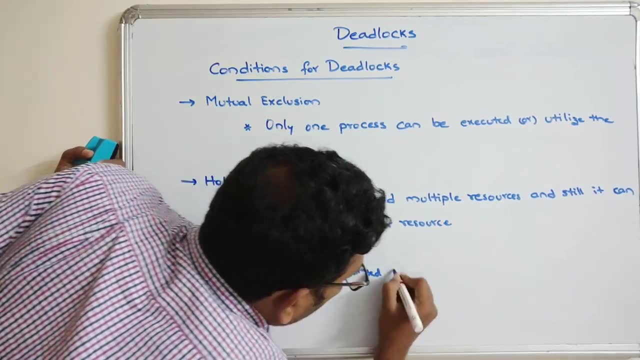 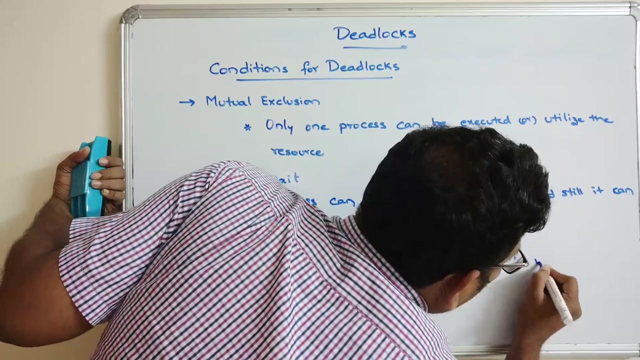 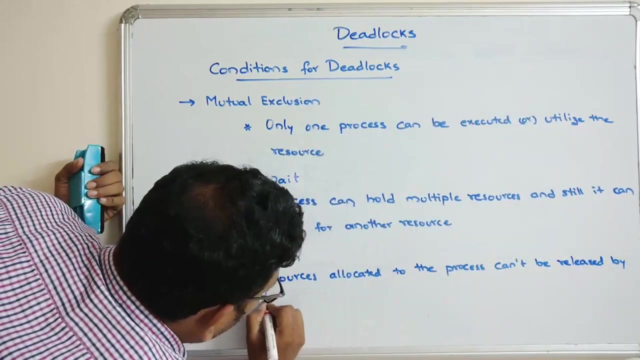 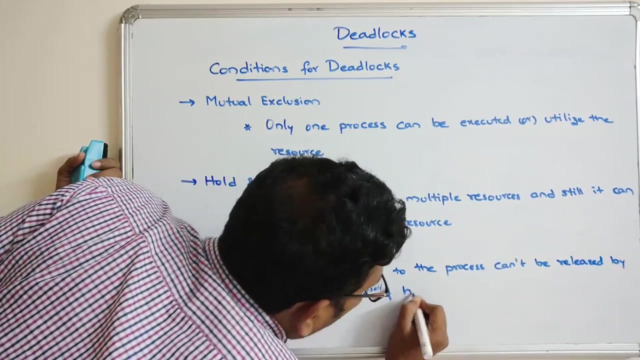 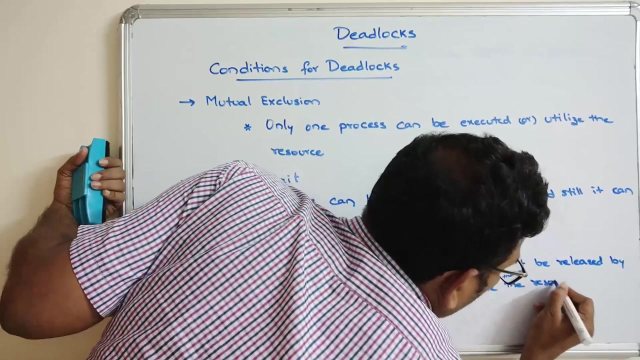 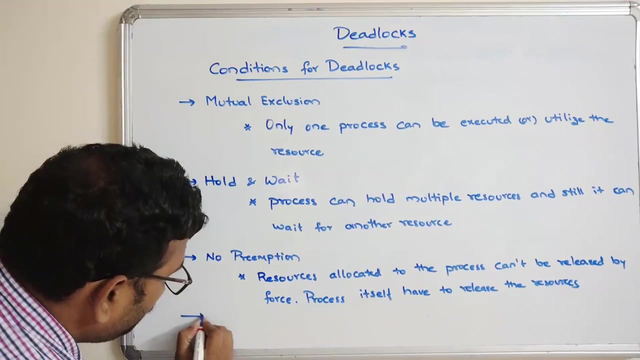 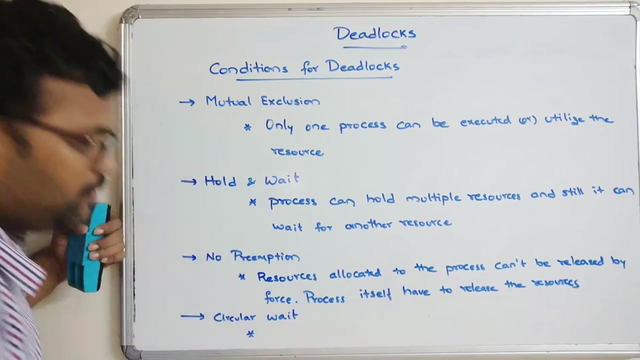 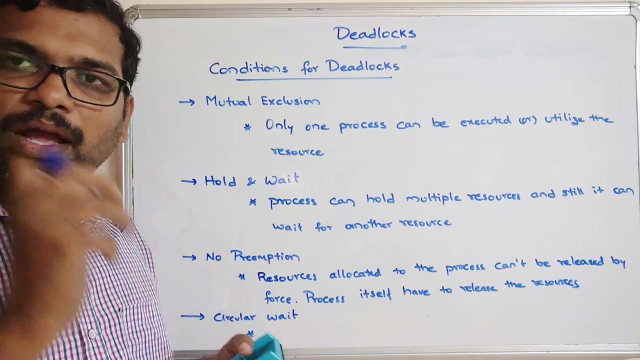 By force, Right. So the resources allocated to the process can't be released by force. Process itself, Process itself have to release the resources. Only the process can deallocate the resources. Okay, And the fourth condition: circular wait, Circular wait. So here the processes will be in a waiting state, in a circular fashion to allocate. 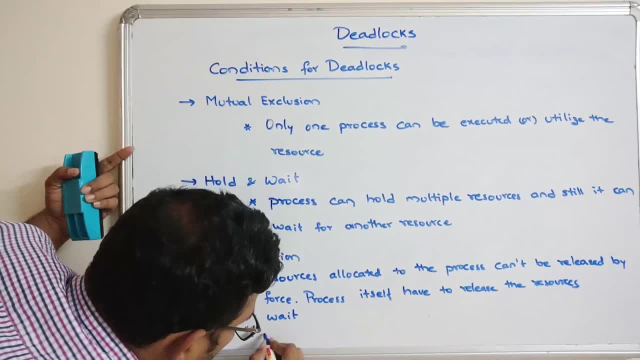 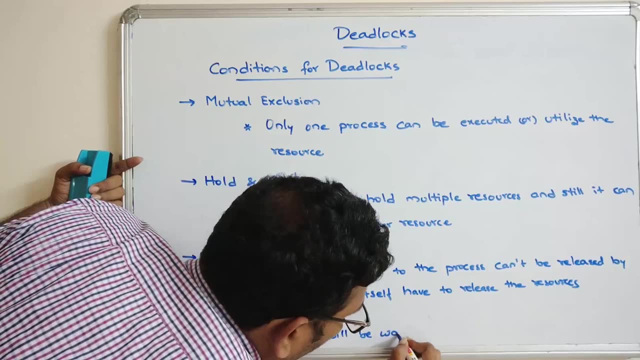 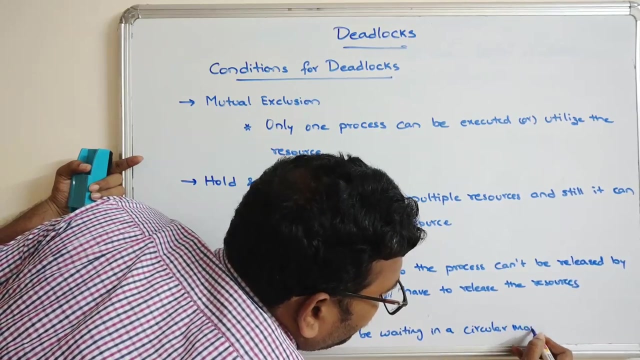 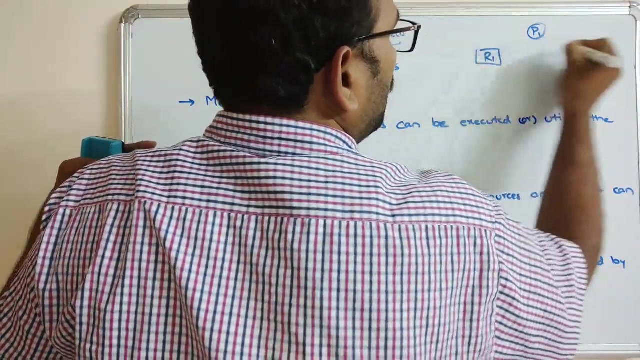 I mean to utilize the resources. So processes will be waiting in a circular manner, Circular manner to utilize the resources. For example, let us take this one: process P1 and resource R1 and resource R2 and process P2.. Okay, 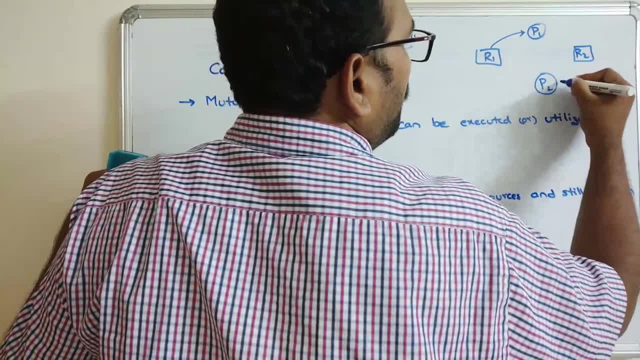 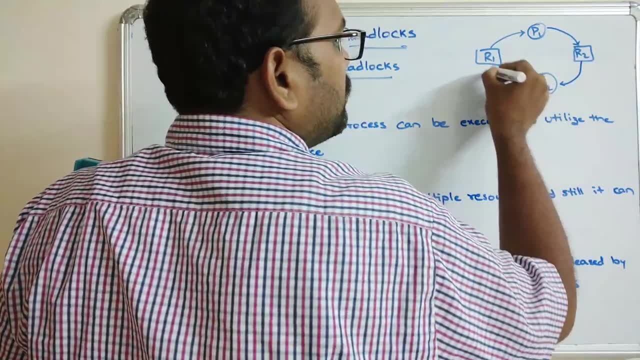 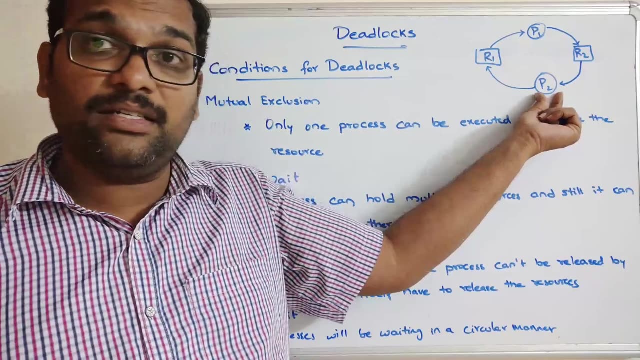 R1 is allocated to P and R2 is allocated to P2.. And see, you can observe P1 is requesting for R2 and P2 is requesting for R1. So you can see the last process is allocated. I mean, the last process is requesting the resource which is allocated for the first process.